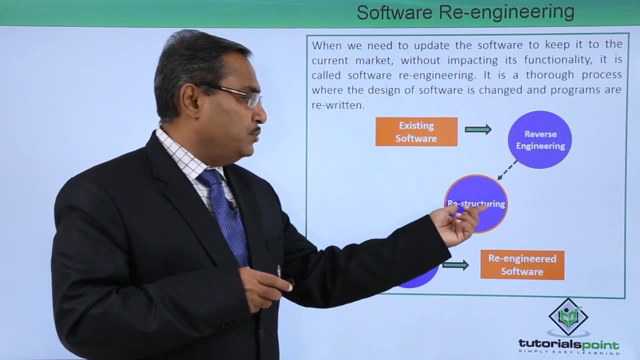 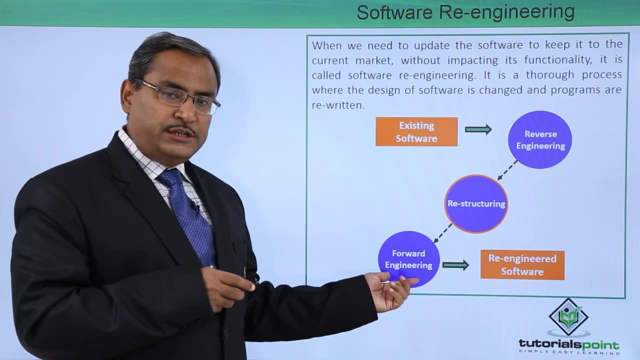 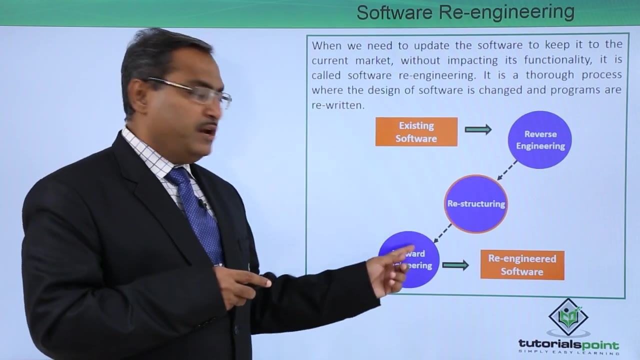 do? We shall go for the reverse engineering and then we shall go for the restructuring of the software and then, from this restructuring of the software, then the forward engineering will take place and then we will be going for re-engineered softwares. So now, here you see. here we are having three different processes. 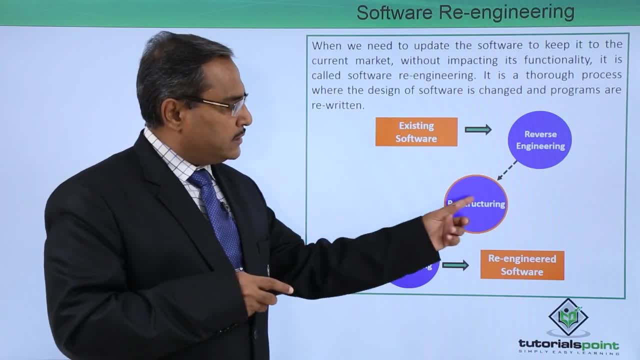 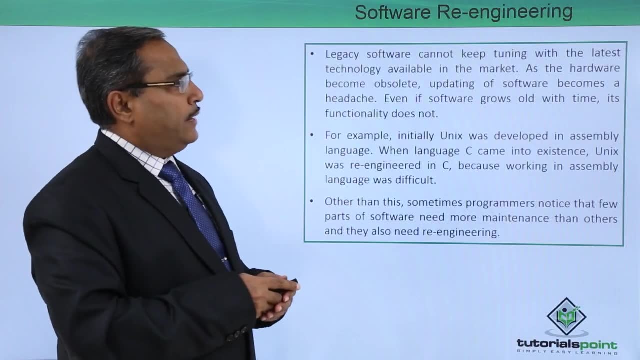 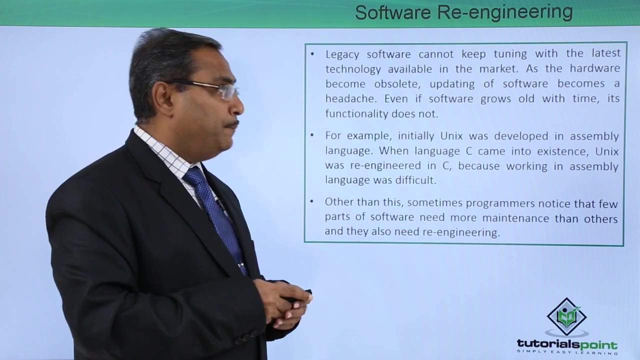 are required to get executed, So we will be discussing three of them in this order in our current discussion. Legacy software cannot keep tuning with the latest technology available in the market, So as the hardware become obsolete, updating of software become a headache. So 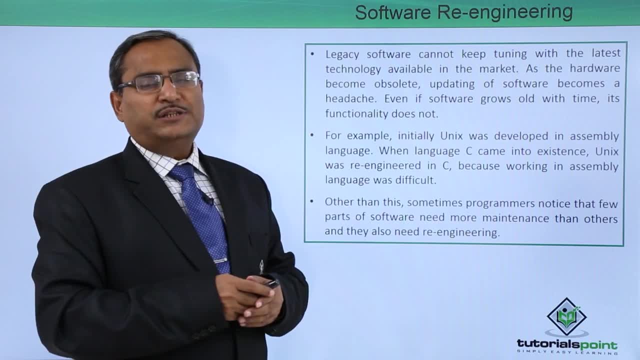 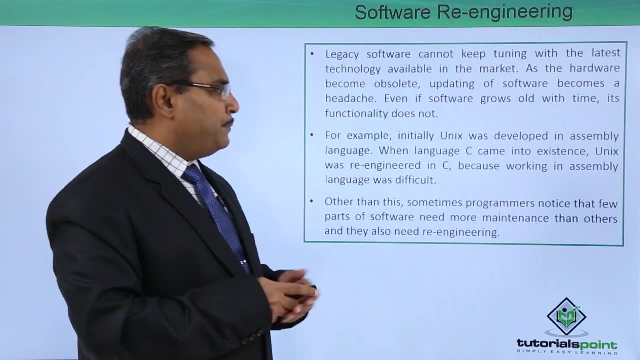 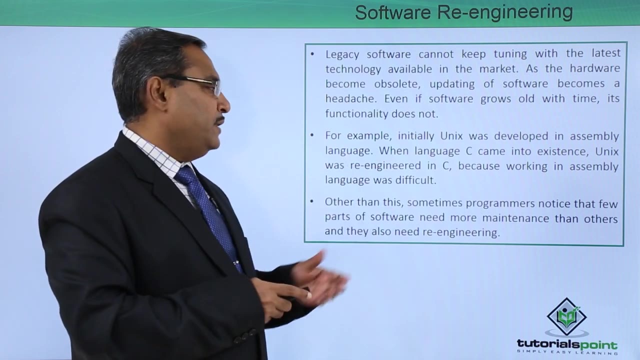 even if the software grows old with time, the functionality does not, and that is the reason for which we require the re-engineering. So, for example, initially Unix was developed in assembly language, but when language C came in the market, into existence, then Unix was re-engineered in C language. and because working in assembly 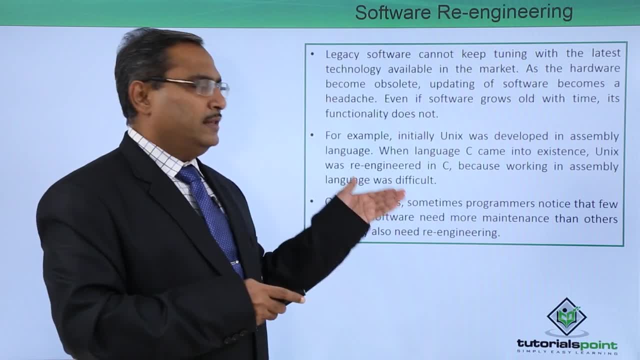 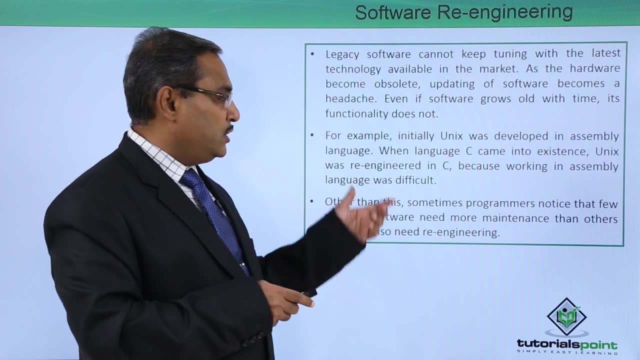 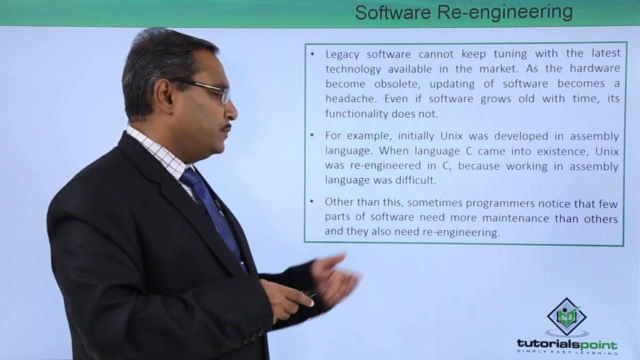 language was difficult. So here you can see that the same Unix which was written in assembly language code, now it has got migrated to this C language and for which we require re-engineering. So other than this, sometimes programmers notice that few parts of the software need. 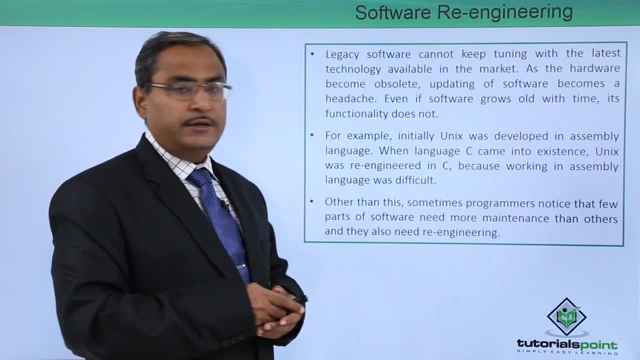 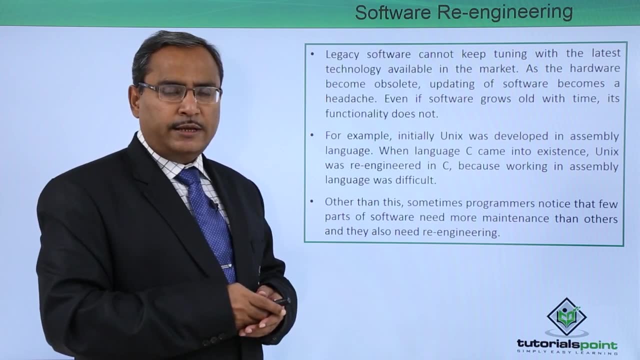 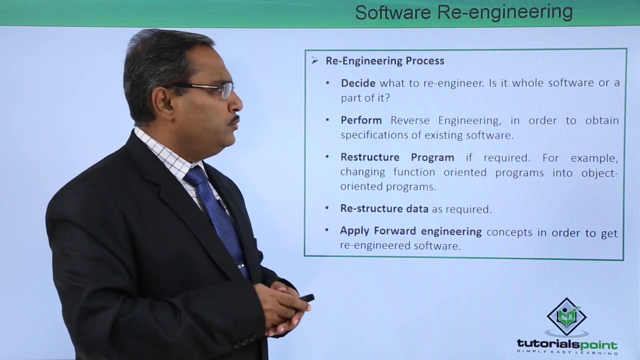 more maintenance than the other, and they also need re-engineering. So these are the different causes for which we have mentioned that, why this re-engineering is required. So now let us go for the re-engineering process, decide what to re-engineer Is it? 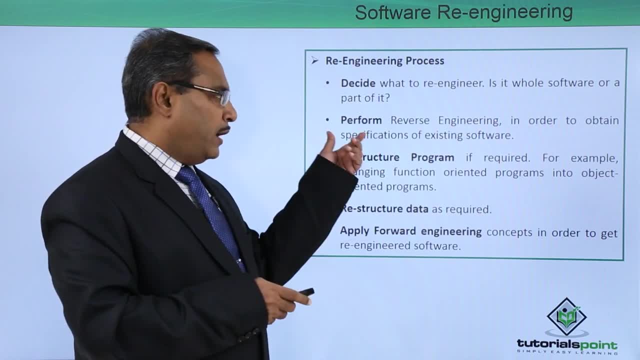 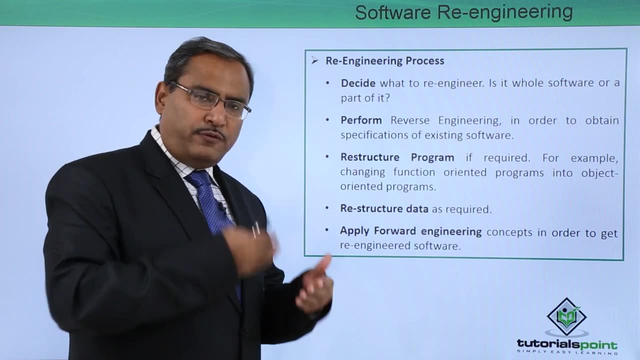 the whole software or the part of it perform reverse engineering in order to, often, the specifications of the existing software. So here we had blank for the reverse engineering, So that from the existing software we are going to get a nice rattling experience with a type of mapping for the difficult and difficult. 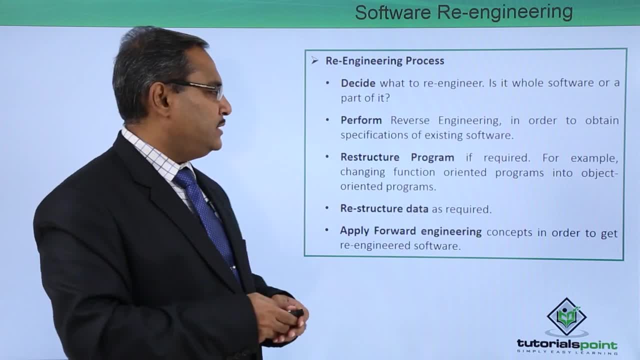 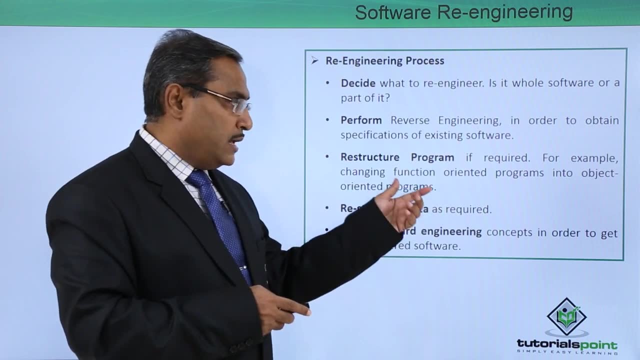 bikes in the software. So this is the reasons for the many components that we need to Planning. we are going to get our specification list. So restructure program if required and, for example, changing functions oriented programs into object oriented programs. So if we require, 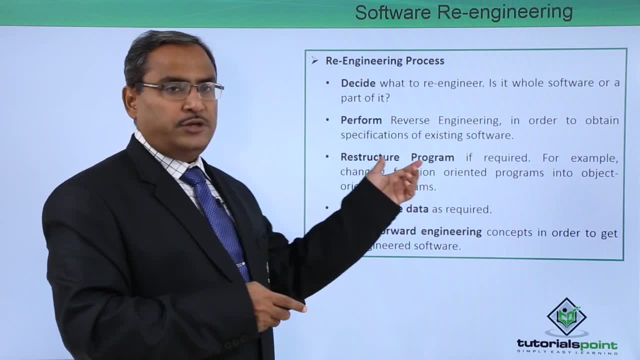 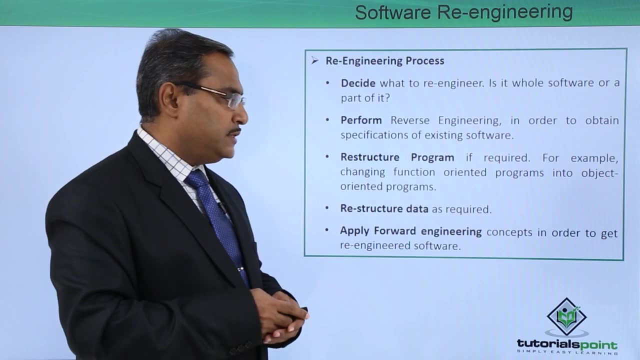 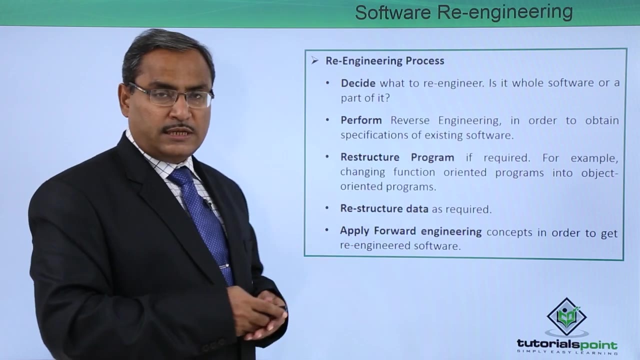 then you can go for some changing in the restructuring of the program, Then restructure data as required and apply forward engineering concepts in order to get the reengineered software version. So in this way, these are the different processes which are taking place in our reengineering. 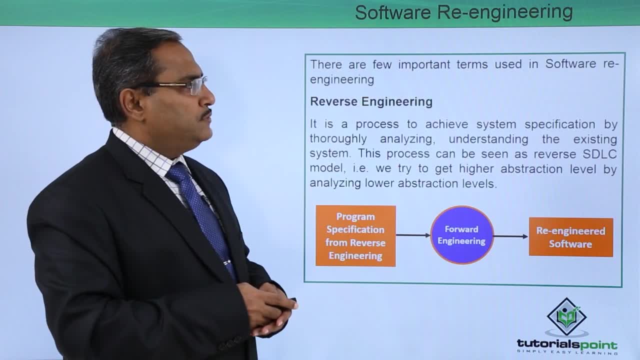 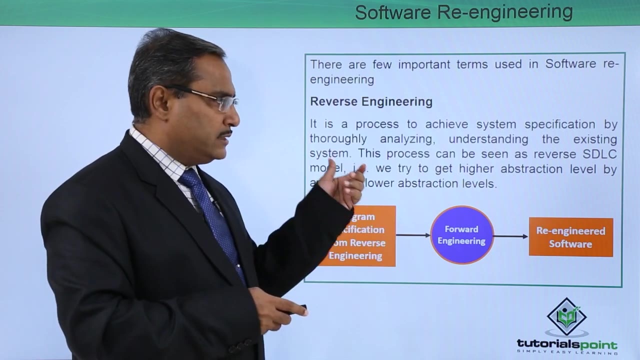 So there are few important terms used in software reengineering, So let us go for one by one. So at first we are going for reverse engineering. So it is a process to achieve system specification by thoroughly analyzing, understanding the existing system. 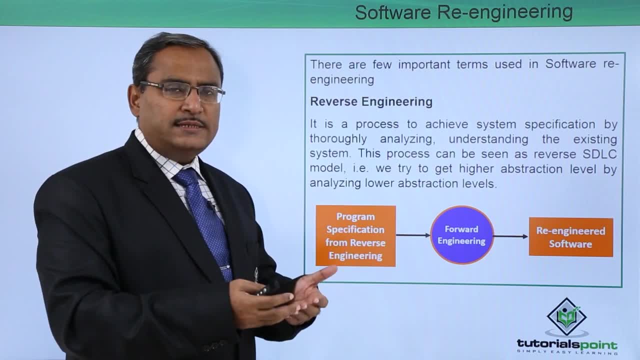 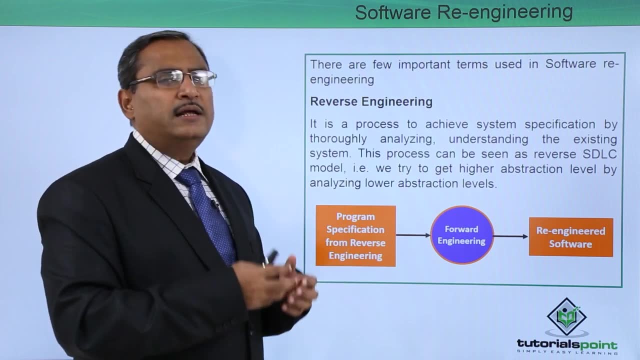 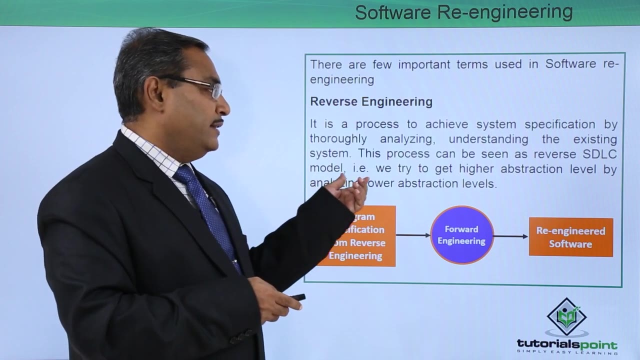 So we discussed earlier also. So from the existing system we are trying to do some understanding, we are trying to do enough and dedicated analysis so that we can get the specification list. So this process can be used as reverse SDLC model, That is, we try to get higher abstraction level by analyzing the lower abstraction level. 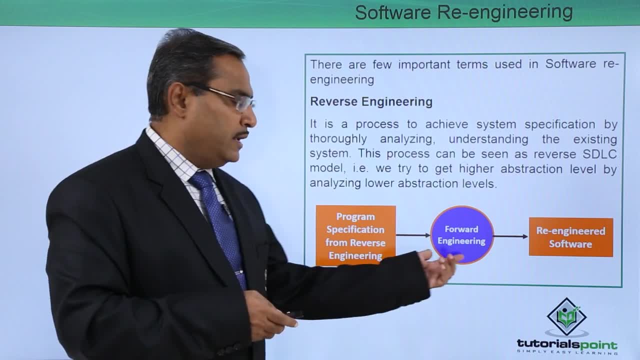 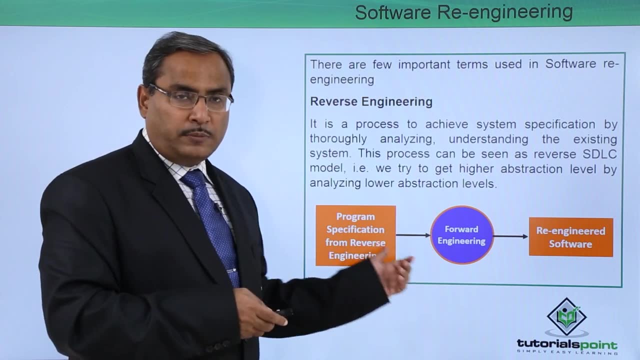 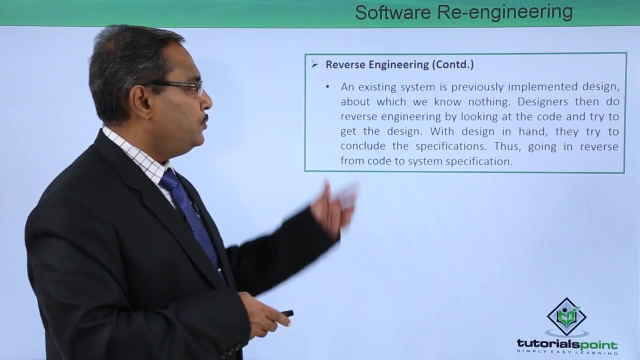 So program specification from the reverse engineering. Now the forward engineering will come and the reengineered software version will be obtained. So that is a part. that is a part of the diagram which you have shown earlier in this video. So now we are going for the reverse engineering continued And an existing systems is previously. 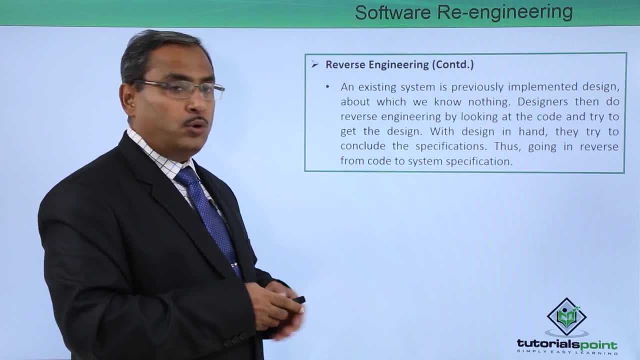 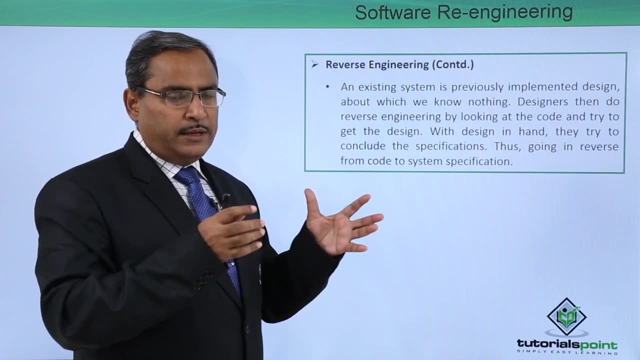 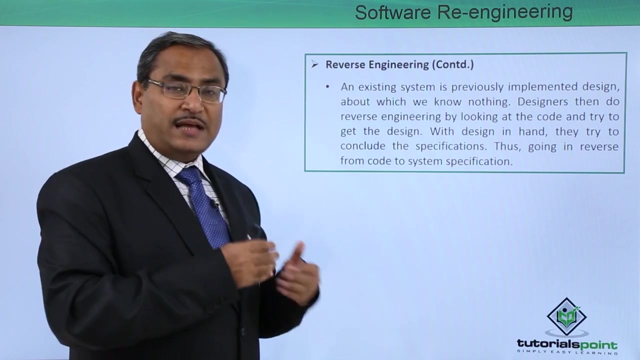 implemented. design about which we know nothing, So an existing system is previously implemented. design about which we do not have any documentation, old documentation. We do not know, do not have any idea, So that is why this is a very challenging one for us. So, designers, they do reverse. 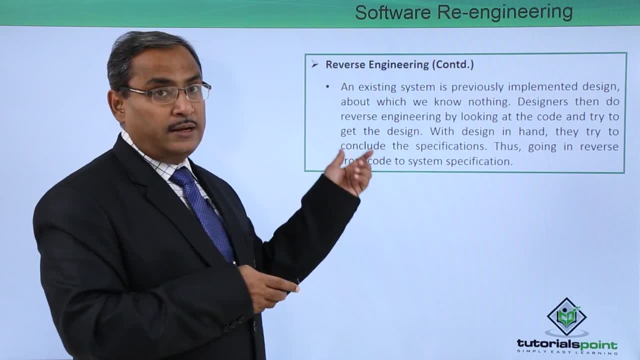 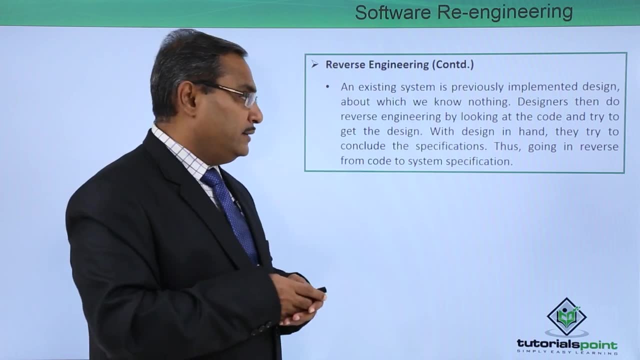 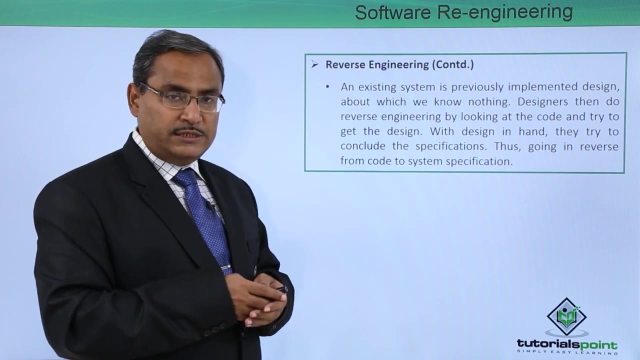 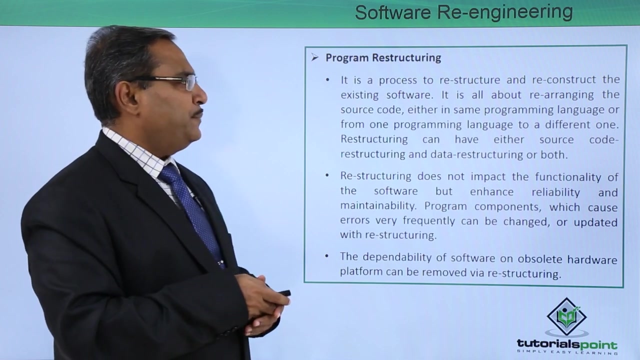 engineering by looking at the code and try to get the respective design While design in hand, then try to conclude the specifications also, Thus going in the reverse from the code to the system specification, and that is the main purpose of this reverse engineering. Next one, the next phase: whatever we discussed was program restructuring, So it is a process. 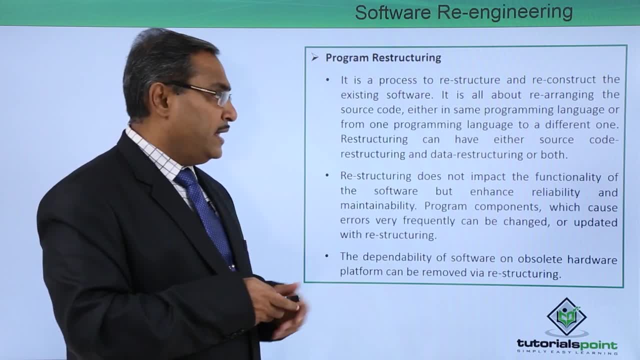 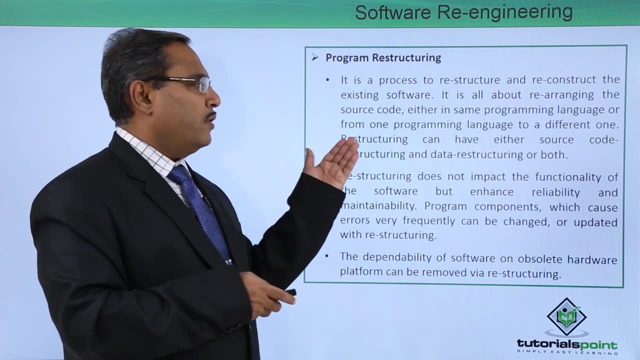 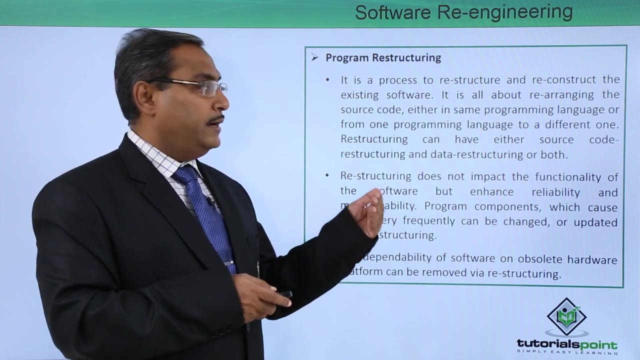 to restructure and reconstruct the existing software, And it is all about rearranging the source code, either in the same programming language from, or from one programming language to another different one, as we had the example of UNIX, where we had to migrate from the ASIM.